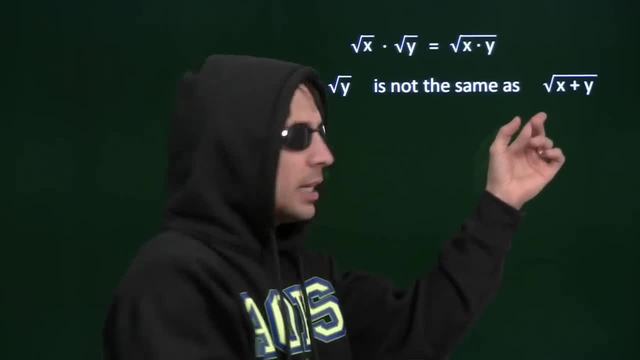 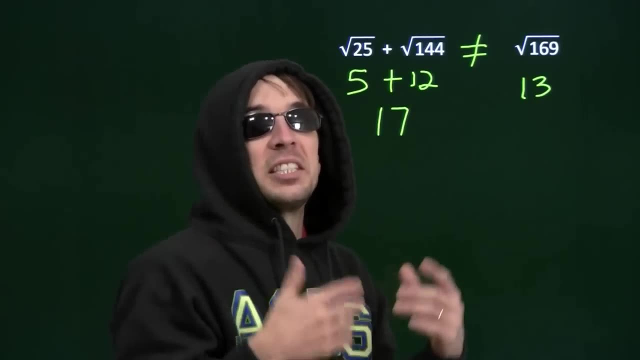 Got that. The sum of square roots is not the same thing as the square root of this sum, because 17 is not 13.. All right, say it with me: 17 is not 13.. So the sum of these square roots is: 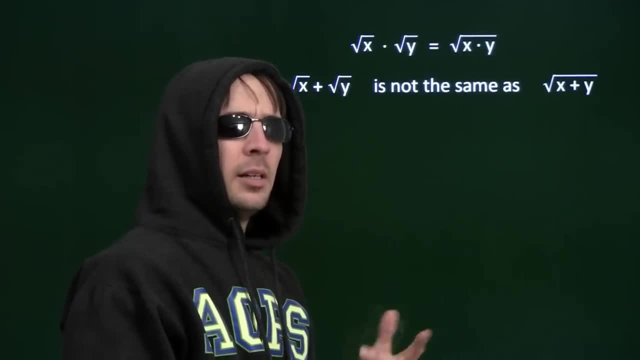 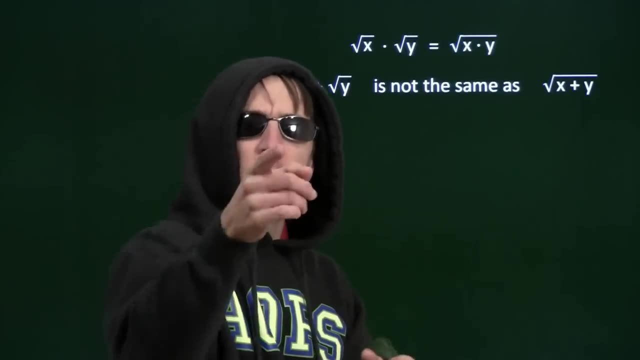 not the same thing as the square root of this sum. You know, I don't think you really have this down, So you know what I'm going to do. I'm going to make you watch me write it down. other guy And other guy. I want you to write it down while you're watching me write it. 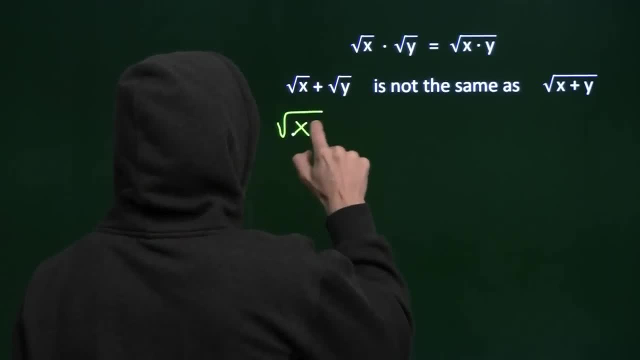 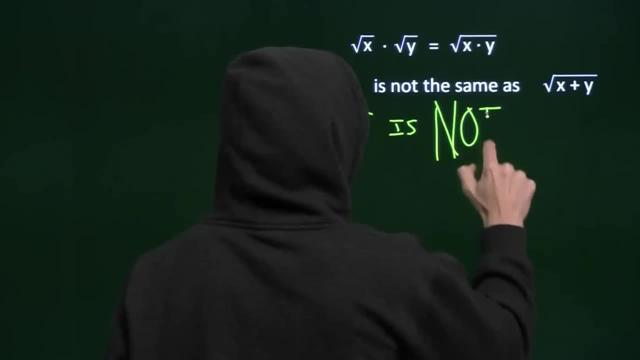 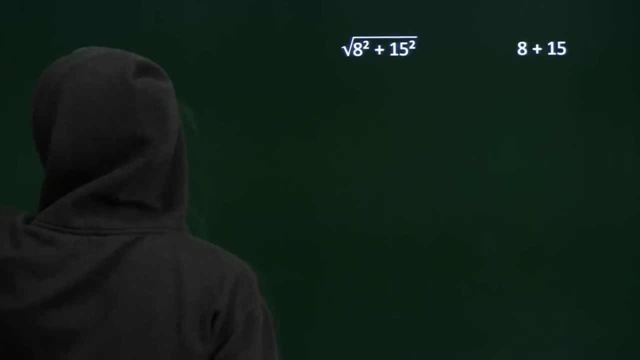 down. So remember, here we go: Square root of x plus the square root of y is not the square root of x plus y. All right, got that Good. All right, let's go on to one more mistake that I don't want you to make when you're teaching the students. Here we go, We got. 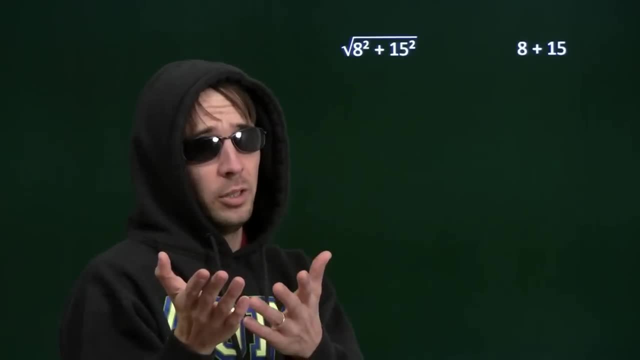 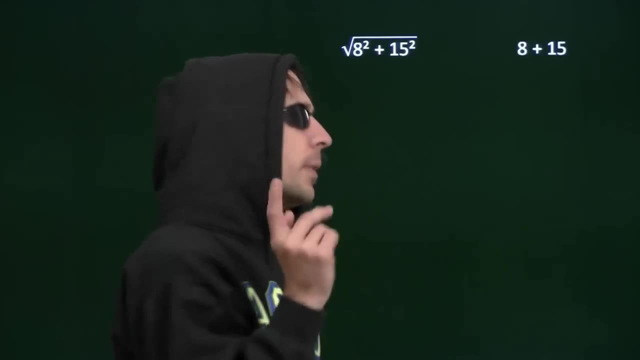 the square root of the sum, a squared plus 15 squared. I know what you want to do. I know you want to say: hey, the square root of 8 squared is 8, and the square root of 15, so these two are equal. 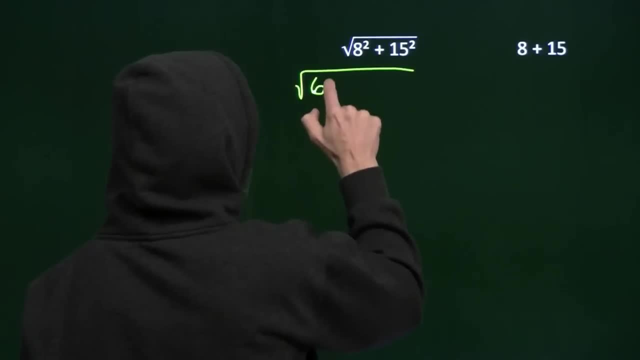 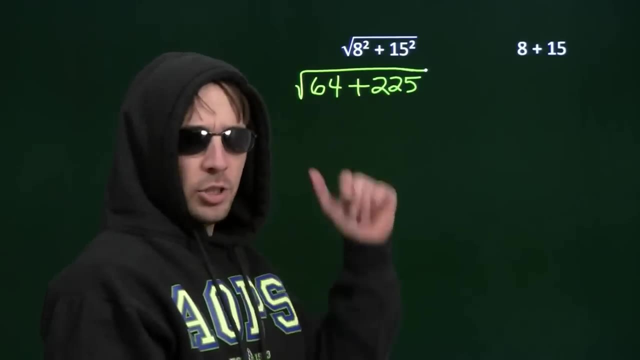 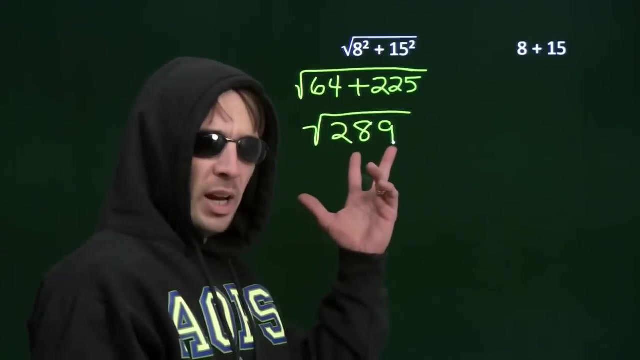 Let's check it out. We can compute both of these squares. we get 8 squared is 64,, 15 squared is 225.. Then we add those two up, we get 289, 64 plus 225 is 289, 289 is 17 squared square root. 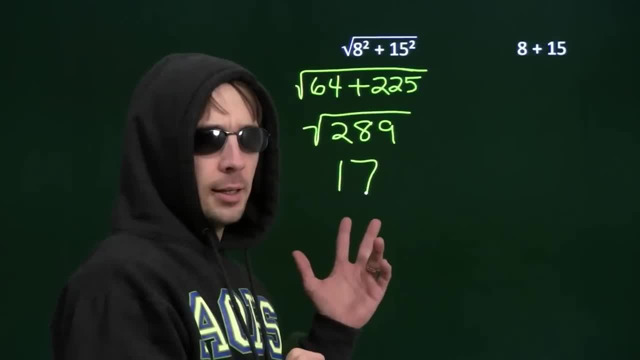 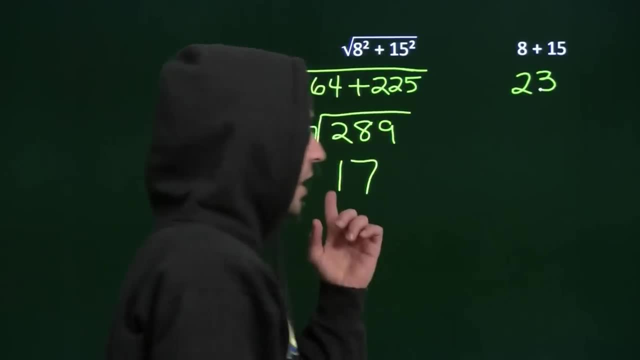 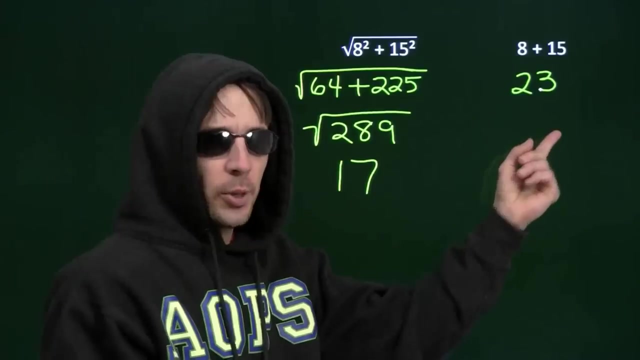 of 17 squared. hey, there's 17 again. Now what do you get over there? That's right, you get not 17,. 8 plus 15 is 23,. 17,, it wasn't 13.. It's not 23 either. 17 is not 23.. 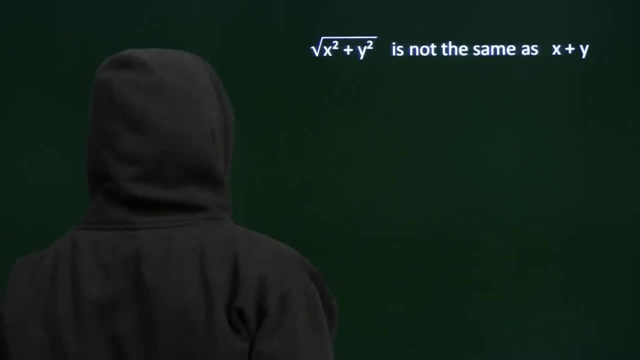 So these two are not equal. And this is what we got here. we got a square root of a sum. We can't just break that up into the square root of the first thing, which here would be x, plus the square root of the second thing, which here would be y. 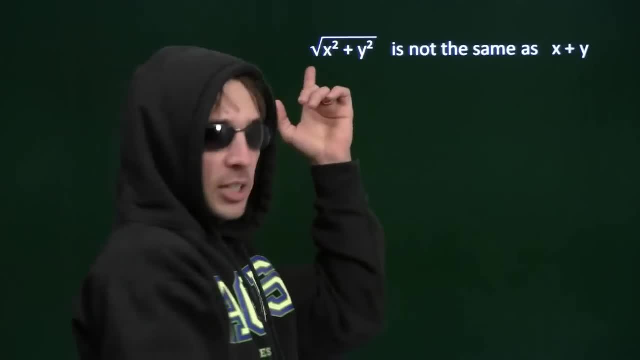 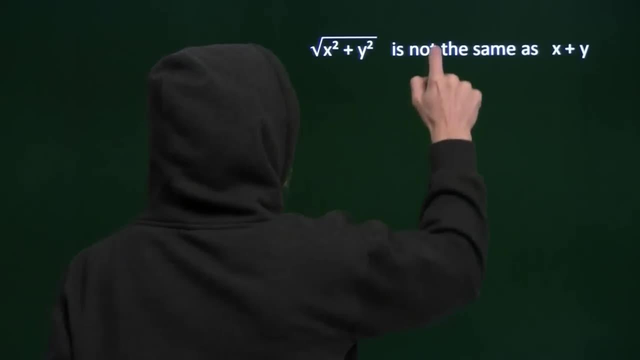 Can't break it up like that. The square root of the sum x squared plus y squared is not x plus y. Got that? You know what? I'm going to make sure you have that. I'm going to circle the not there.